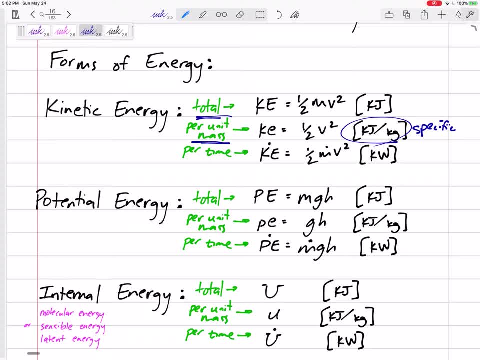 Okay, so a few things you know to look at. It might say specific or total or per time, The units might give it away or these variables in general. Capital is total, Lowercase is specific And if you've got this dot over it right here, that dot is like the derivative. 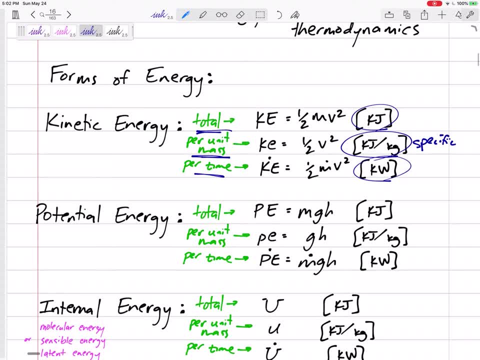 the kind of the per unit time. So total, if we're trying to calculate total kinetic energy, that's one half mv squared. The units are kilojoules. If we are looking at specific, it's just one half v squared. 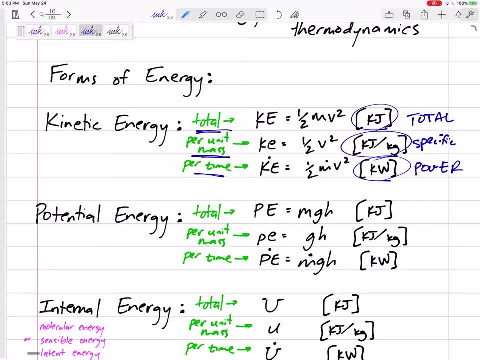 And here this is. This is kind of power, it's kind of work per divided by time, energy per time, And so maybe kilowatts would be our units We need to. we'll kind of go over the units some. 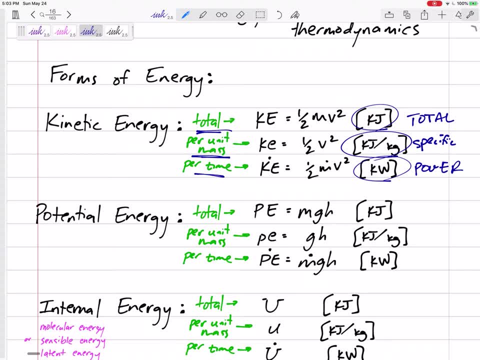 whereas meters per second, quantity squared, you know, is just joules per kilogram. There's some interesting units here: Watt is a joule per second. Okay, so anyway, kinetic energy: One half mv squared if we're looking at total. 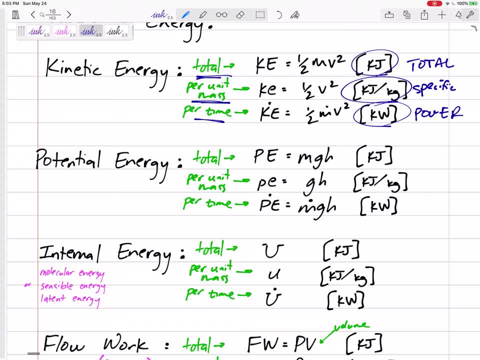 Potential energy total would be mgh. right, mgh is our total potential energy. If it's specific, then it's just gh, And if it's per time, it's m dot gh. We'll talk about this m dot on the next page. 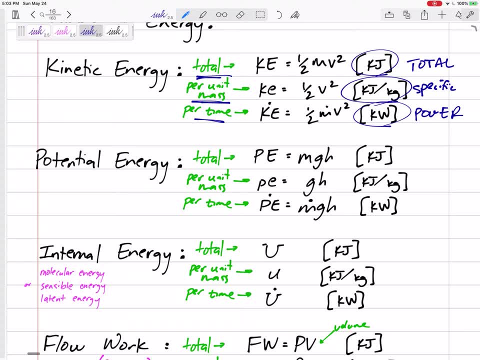 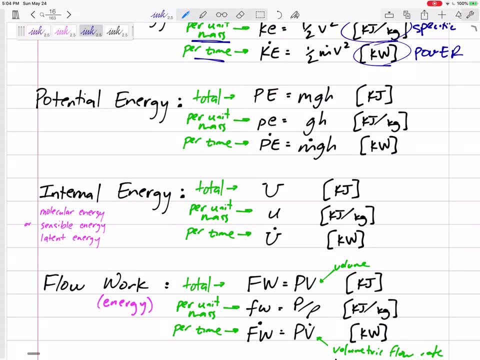 Sorry, right here and there, That's the mass flow rate, That's the mass per unit time. Okay, and then there's internal energy. That That is capital. U lowercase, u or u dot. That's kind of on a molecular level, how much energy is inside of the fluid. 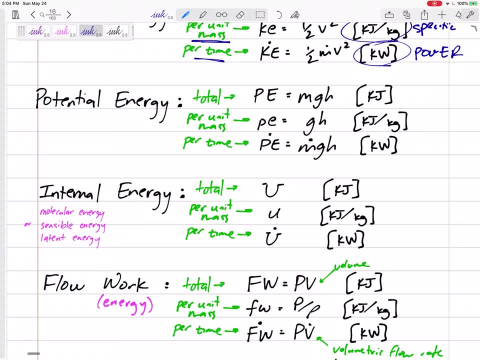 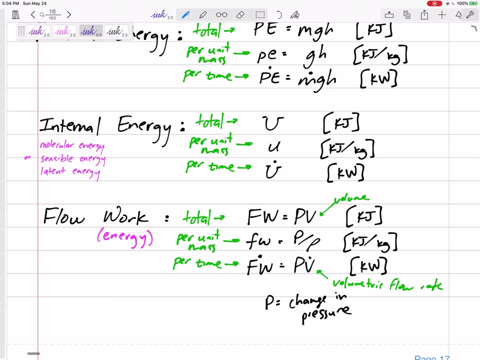 So we won't really calculate that. We won't have a formula for that. In the future we could find that in a property table on the back of our book. And then there's flow work, Flow work. it's pressure times, volume or pressure over rho. 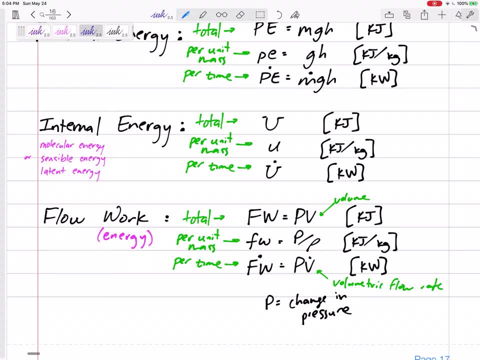 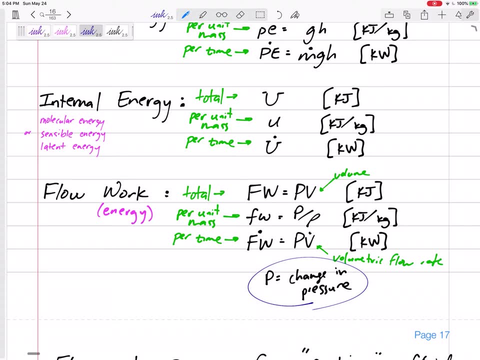 Rho is the density here, Or pressure times, volumetric flow rate. But actually it's not exactly just pressure, It's the change in pressure. It's the change in pressure. If there is no change in pressure, then there's going to be no flow. 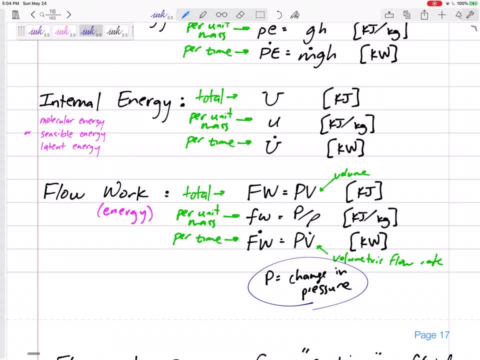 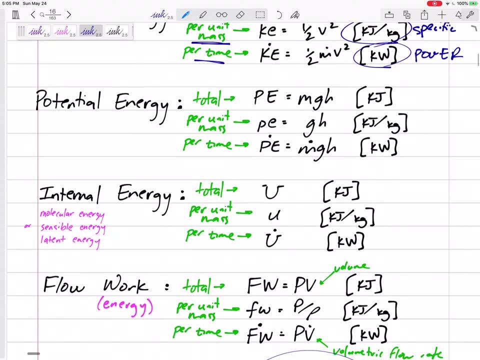 And so that flow work is the change in pressure times, the volume. All right, so anyway, here are four different types of energy that we can be looking at in our problems when we're calculating: hey, how much energy is there? to begin with, 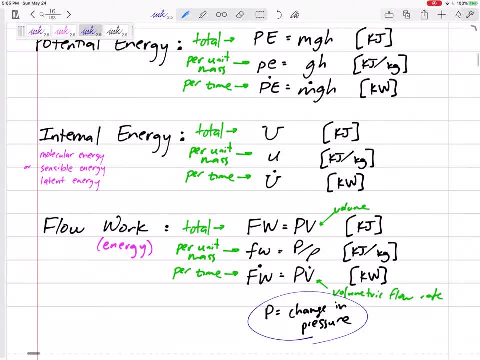 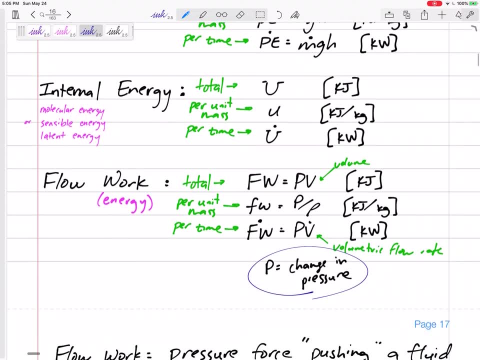 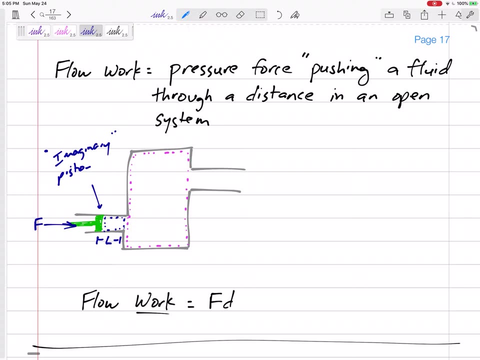 How much energy is there? final, Was there any change in energy? These are the four main types of energy we'll be calculating for now Let's talk about this flow work. Flow work is a pressure force pushing a fluid through an open system. 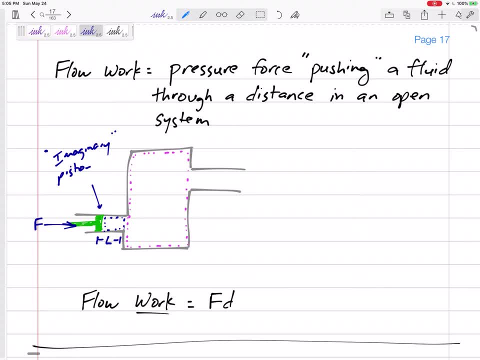 So imagine that we have an open system. We have an inlet and an outlet. Let's pretend like this inlet. In order for fluid to go into the inlet, there needs to be a pressure pushing it into the inlet. So let's pretend like there's some imaginary piston right here that is pushing this fluid in the blue little volume. 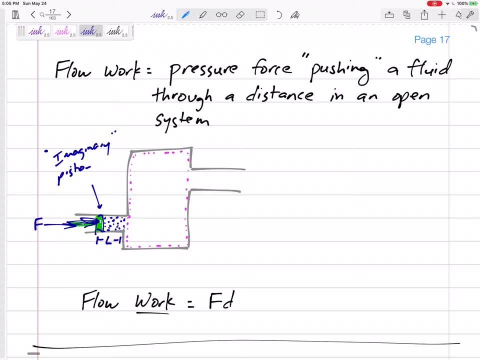 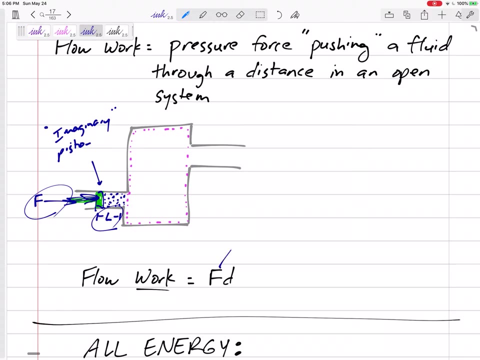 across our boundary into our system. In order for fluid to go into our system, there's got to be a force pushing it And it's going kind of a distance L. This force right here would be. let's see, pressure equals force over area. 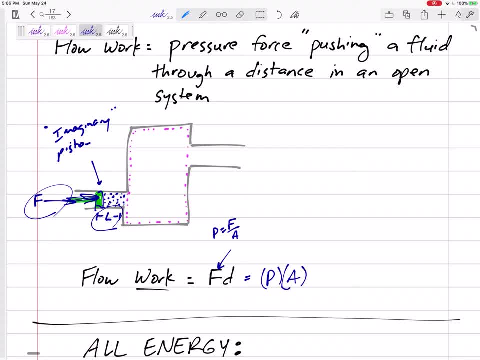 So we could just say a force is a pressure times an area right here, Here the area is the cross-sectional area right here of our inlet. So we're going to say a force is a pressure times an area right here of our inlet, times a distance L. 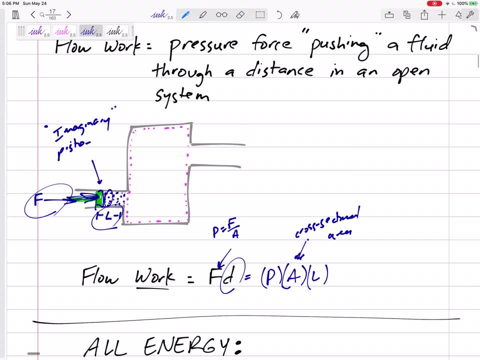 And the cross-sectional area times. this distance in this case would be L. And what is area? cross sectional area times L? that's kind of the volume of the inlet. So here that's why our equation for flow work is pressure, which is kind of a change in pressure. 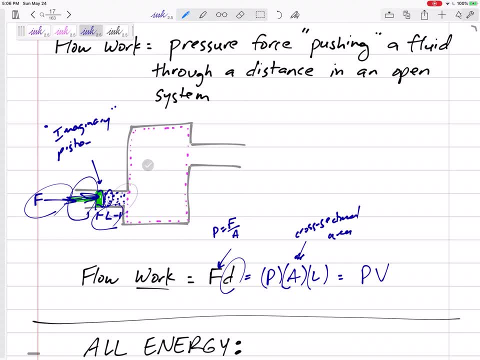 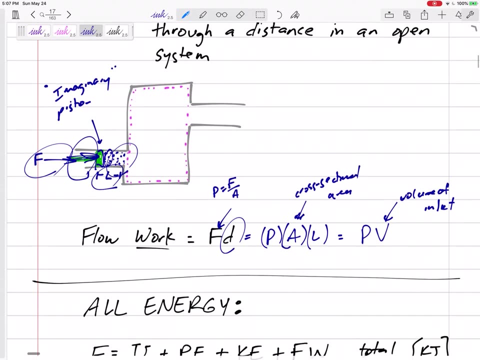 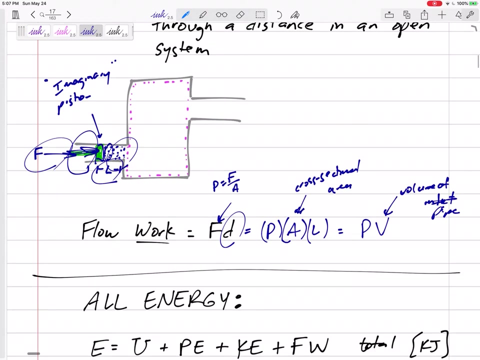 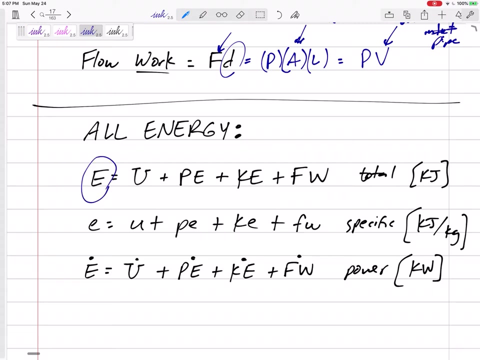 the difference in pressure from outside to inside times the volume, right here. Pressure or change in pressure times the volume, Volume of the inlet, volume of that inlet or that pipe, let's say that pipe right here. Okay, so anyway, if we want to calculate all the energy, all the total energy, capital E. 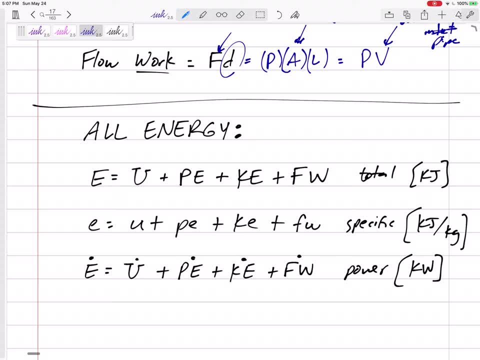 then we would add up the internal energy plus potential energy, plus kinetic energy, plus the flow work. If we wanted to calculate all the specific energy- lowercase letters- we'd add up all the internal energy, potential energy, kinetic energy, flow work, specific. 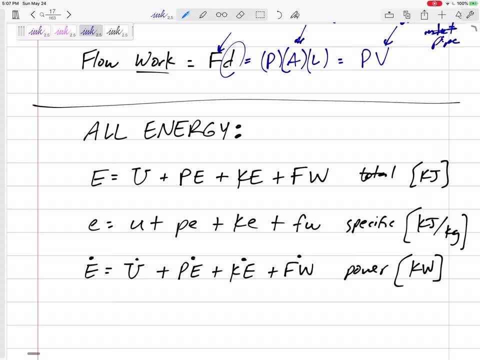 And if this was a power type of problem, if we wanted to calculate all the power of our system or maybe the change, then we would have these: capital, the mass rate of change, the per unit and the time of potential energy, kinetic energy, flow, work and internal energy. 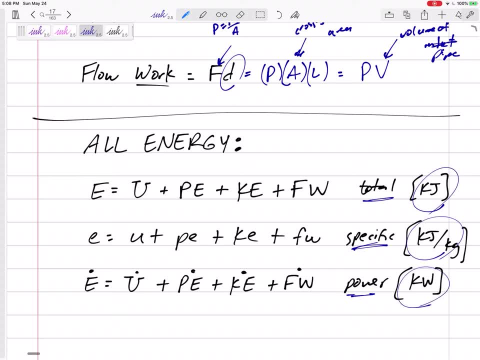 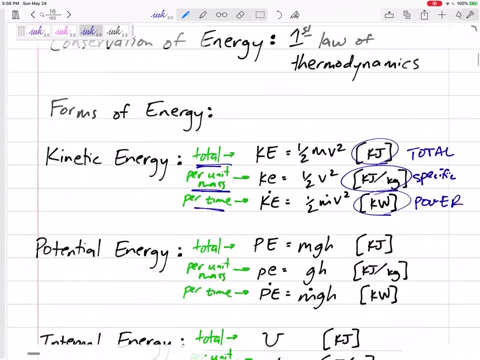 But look for these keywords, look for these units, look for these capitals and lowercase and mass flow rates to kind of make sure you're using the right equations, using the right formulas. Okay, now remember this m dot. we haven't talked much about that. let's talk about that. the mass flow rate. 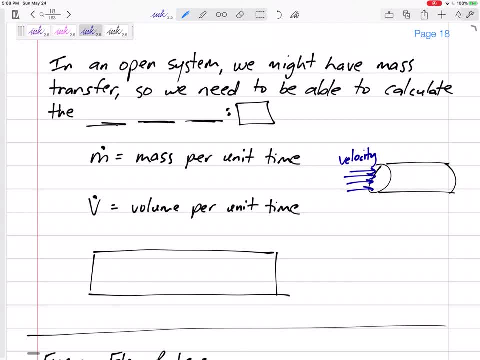 Because in an open system we might have mass going into and out of our system. so we need to calculate the mass flow rate. mass flow rate, the m dot. We need to calculate the m dot. This is the amount of mass flowing per time. 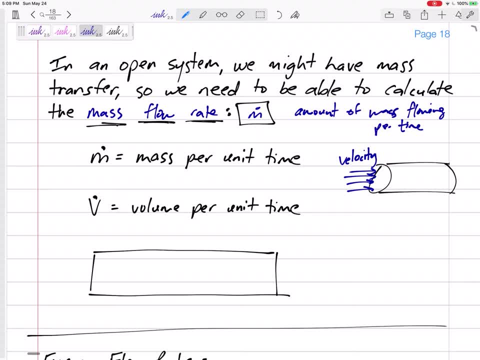 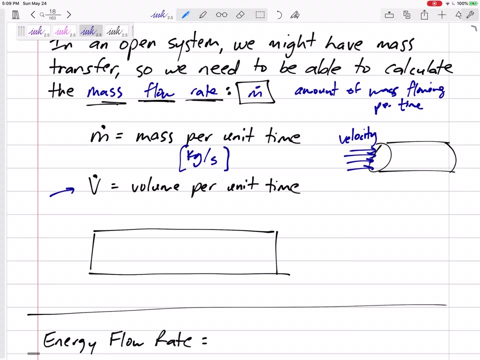 This is the amount of mass flowing per time. mass per unit time. The units for m dot would be kilograms per second right. The units for mass flow rate would be kilograms per second. Now we also might want to calculate the volumetric flow rate. 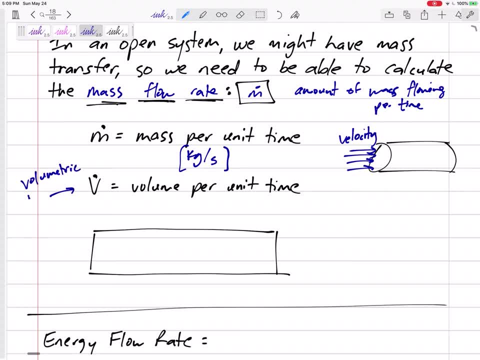 This is the volumetric flow rate, capital V dot, and that would be the volume per unit time. m cubed, divided by seconds, would be the units for that right. How much vol? what's the volume? What's the volume of fluid that is entering my system per unit time? all right, 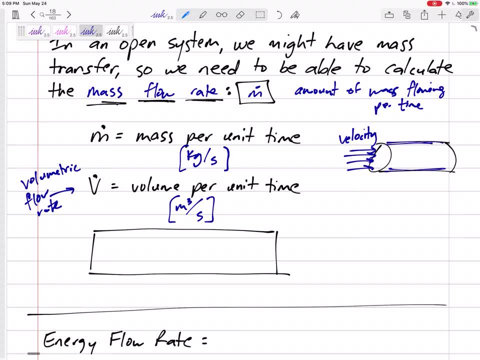 So you know, imagine you've got some inlet, some pipe and you've got fluid going through here at some velocity. We want to keep track of how much mass is coming in, or maybe we want to keep track of how much volume is coming in. 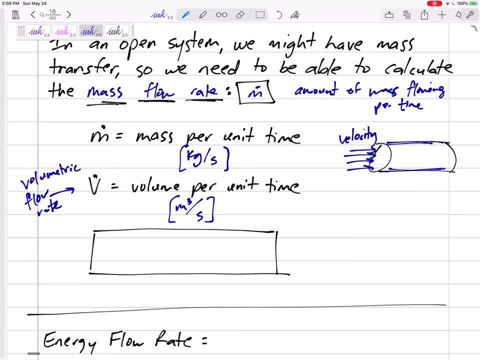 Or really, you know, our equation calls for an m dot. We need the m dot. Our equation calls for a volumetric flow rate. We might need that. Are these related? Are these related? Probably, and they look kind of similar. 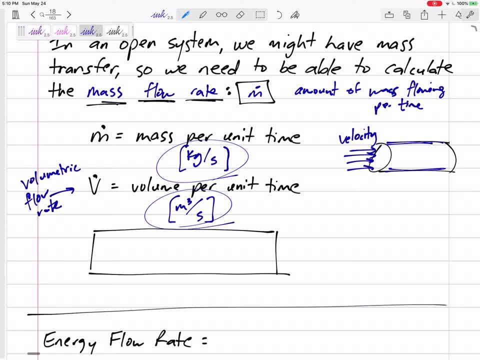 Instead of kilograms per second we've got meters cubed per second. How could we kind of convert between mass flow rate, volumetric flow rate? Are they related? Units would give me a clue here. They are related by density, right. 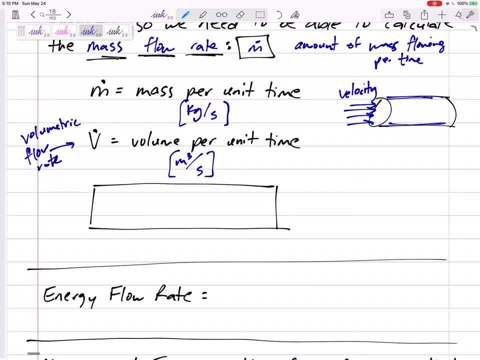 They're related by density. Does it make sense- Let me see this- That m dot Density would be equal to rho times v dot. m dot would be equal to rho times v dot. Let's see if the units work out here. 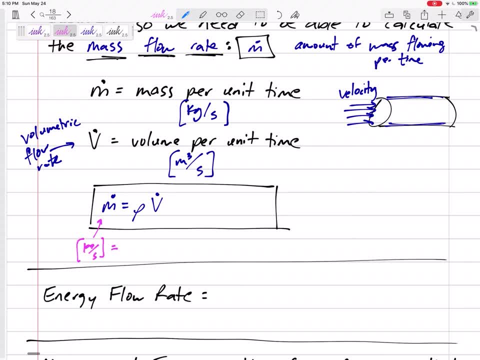 Kilograms per second is the same as what is density. Density is kilograms per meter cubed. Yeah, and meters cubed per second- Yeah, that works out. That is a great formula right here to know off the top of your head. 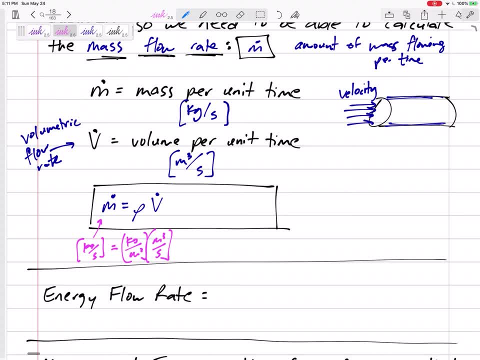 Or you know to have on your. I've kind of mentioned that on the test you'll be able to write your own 3 inch by 5 inch index card, front and back, full of equations. That's one, but you should know that. 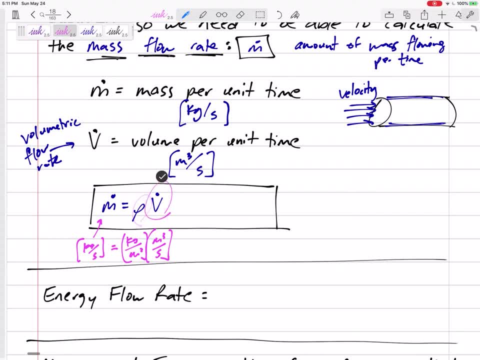 You should have that memorized So you know, for instance, if they give us the v dot and the rho, then we've really got the m dot, We've really got the mass flow rate. Now, if we thought about and looked at this volumetric flow rate, 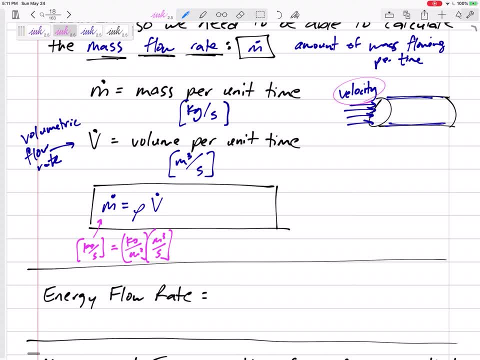 it's related to the velocity. It's related to the velocity. Let me think about this. The volumetric flow rate that has units of meters cubed per second. Our velocity is going at a meter per second If I take the velocity, which is kind of a length per second. 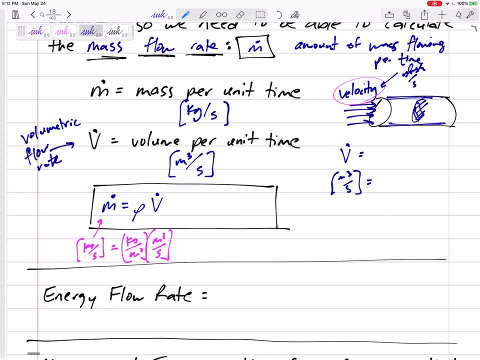 and multiply. I thought about Multiply this cross-sectional area, The volumetric flow rate would be equal to the velocity times the cross-sectional area. The units: meters per second area, meters squared. The units work out, And thinking about this: length times the cross-sectional area. 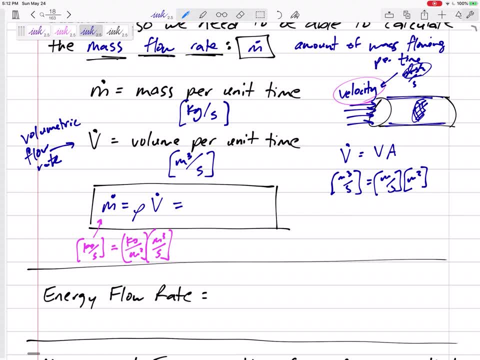 that kind of is the volume. So we can kind of extend this Rho V A. Okay, but be careful This time. this V is the velocity, all right, Okay. so sometimes you know we're looking for the mass flow rate. 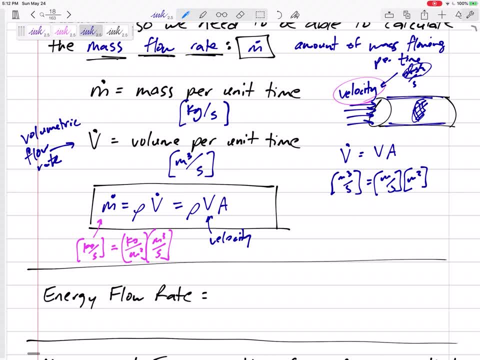 Maybe we've got an equation that we need the mass flow rate, We need the m dot. But the book, being mean, doesn't tell us the mass flow rate. but it does tell us the cross-sectional area of the pipe. It does tell us the average velocity of the fluid in there. 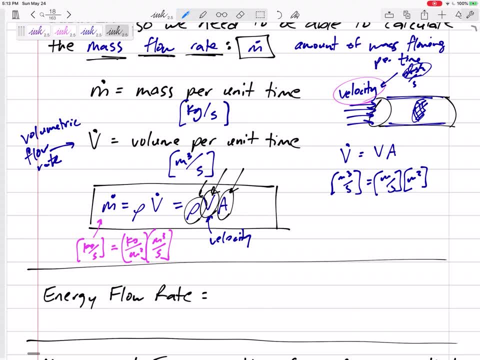 We know the rho of the fluid. Okay, We use those. We use those right to get the mass flow rate so that we can do 1F, m dot V squared, if that's what it calls for, or m dot G H, if that's what it calls for. 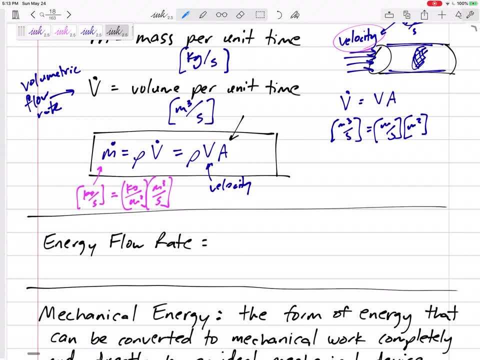 Okay, Okay, energy flow rate. If we want to find the energy maybe flowing into our system per second or per unit time, like E, dot, m dot times or case E, the specific energy, specific energy times, the mass flow rate would give us the energy flow rate. 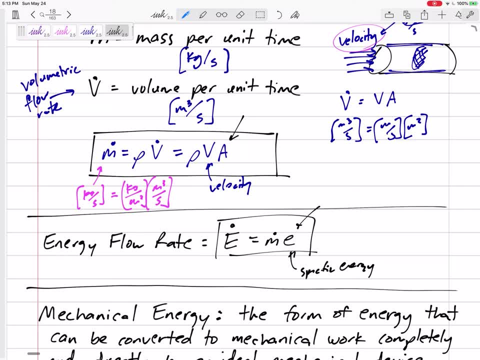 So you know again, if we're given this specific energy, multiplying it times the mass flow rate gives us the energy per unit time or the energy flow rate. We can look at the units: Units. units this class more than. 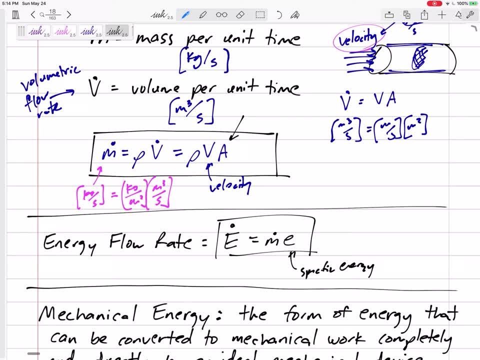 any of the others I teach. Units are maybe a little bit more difficult, but they're definitely a lot more helpful. The units will help us make sure we're on the same page, make sure we are answering what we're trying to find. 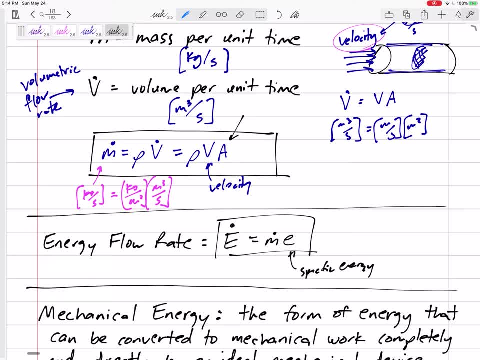 Answering what we're trying to find. Okay, This energy flow rate is kind of a power that would have units of watts or kilowatts. I don't know if I've mentioned before, but a watt is a joule per second. 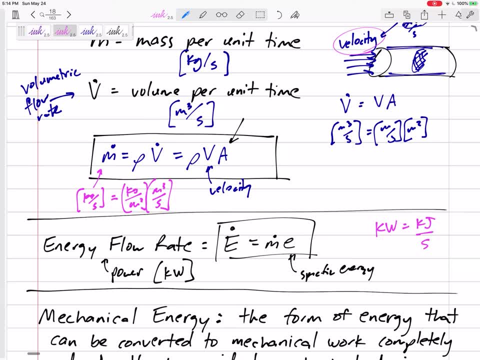 a kilowatt is a kilojoule per second, right here. So if we look at the units, mass would be kilograms per second. Energy is kilojoules per kilogram. Yeah, kilojoules per second, we'd be in kilowatts. 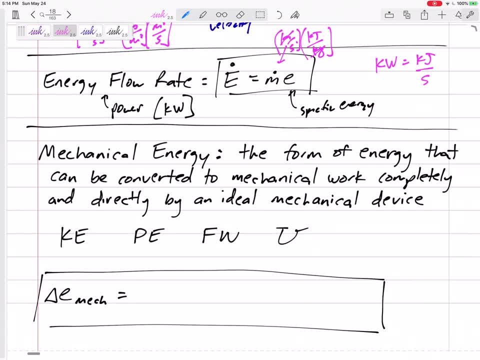 Okay, And then, lastly, mechanical energy is the energy that can be converted to work completely And directly by an ideal mechanical device. All right, We can convert kinetic energy into work. We can convert potential energy into work. We can convert flow work into work. 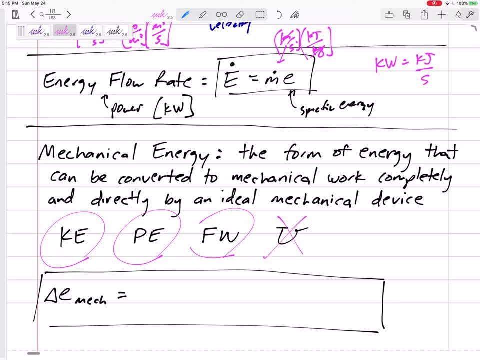 But here we go, You of the energies we've talked about up to this point, those four energies on the first page of this chapter. internal energy is not a part of the mechanical energy. All right, We can't convert Internal energy completely into work. 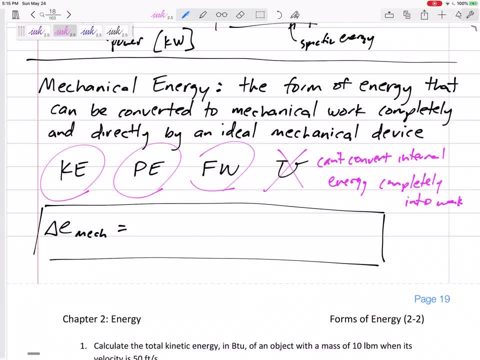 So if it asks for the change in mechanical energy, or if we're trying to calculate how much work we could get out of a system if this was the change in lowercase e: all right, lowercase. so this is specific, All right. 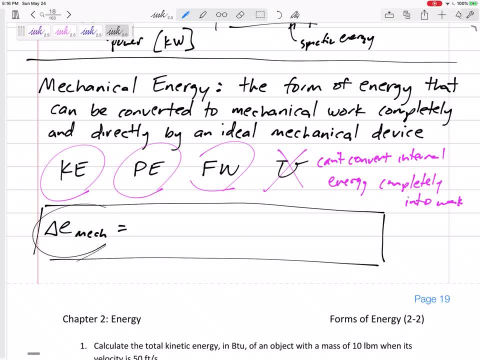 Let's see here: If we want to find the change in mechanical energy, then we need to find the change in kinetic energy, which is one half V2 squared minus V1 squared, or V, you know, final squared minus V, initial squared.